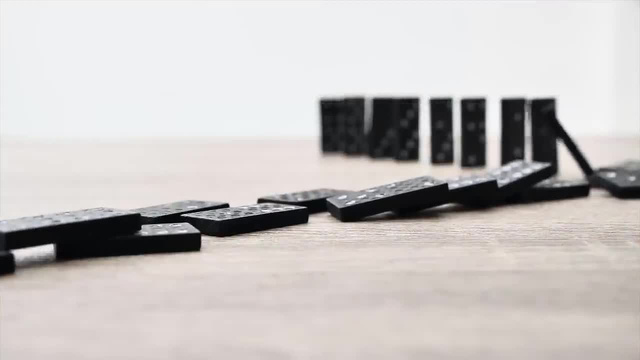 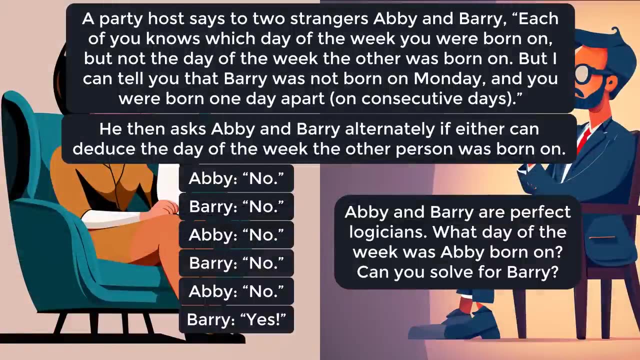 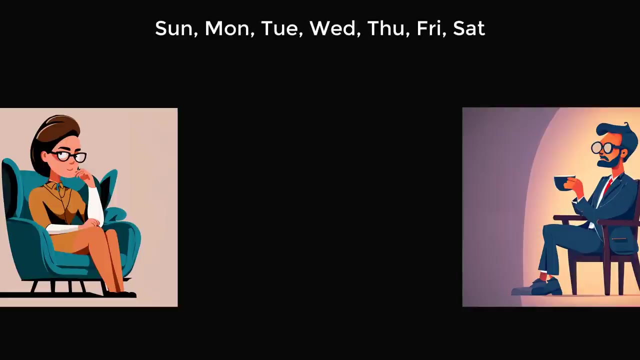 You start out with one deduction and that leads to the next deduction until you keep going and topple down all the dominoes. So how are we going to solve this problem? There are seven days of the week: Sunday, Monday, Tuesday, Wednesday, Thursday, Friday and Saturday. 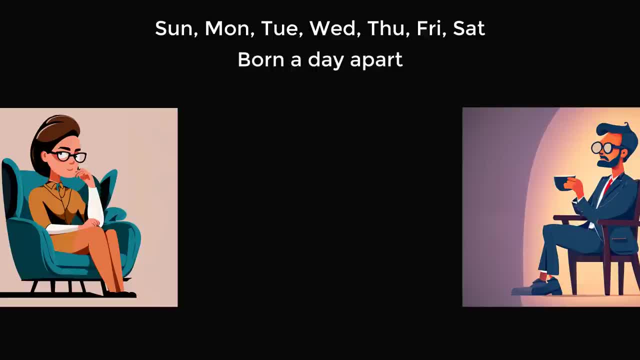 Abby and Barry are born a day apart, So there are 14 possibilities for the days that Abby and Barry could be born at. Let's write each possibility as an ordered pair: Abby comma- Barry. If Abby were born on Sunday, then Barry could be born on the next day, which would be Monday. 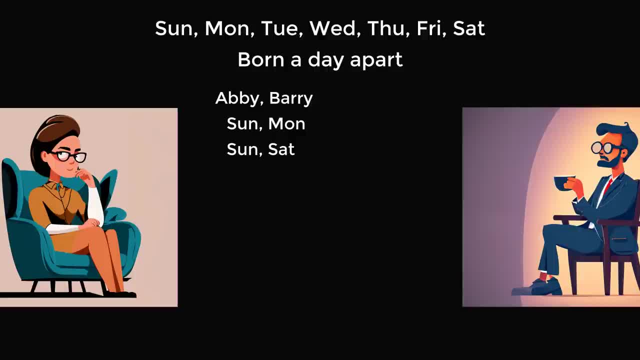 or Barry could have been born on the previous day, which is Saturday. So the two possibilities are Sunday, Monday or Sunday- Saturday. If Abby were born on Monday, the two possibilities would be Monday, Sunday or Monday- Tuesday. Let's write out each of the possibilities for every single day of the week. 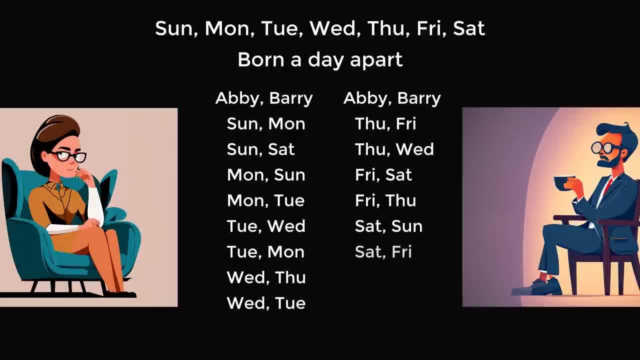 There'll be a total of 14 possibilities. Now what is the first domino in this puzzle? The host says that Barry was not born on a Monday, So we can look at the options where Barry is born on a Monday and we can eliminate them. 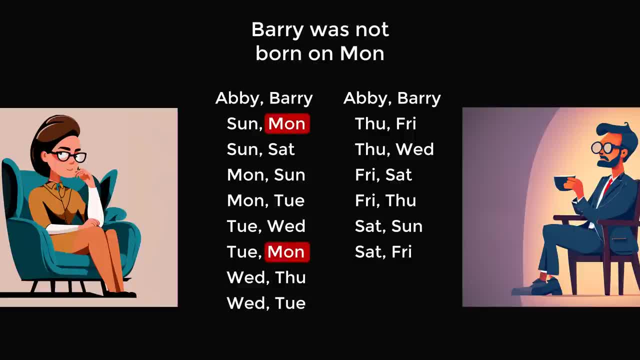 So this will be Sunday Monday or Sunday comma Monday, or it could be Tuesday comma Monday. Now Abby says no. I still cannot deduce which day of the week that Barry was born on, So this will be the next domino that falls. What information. 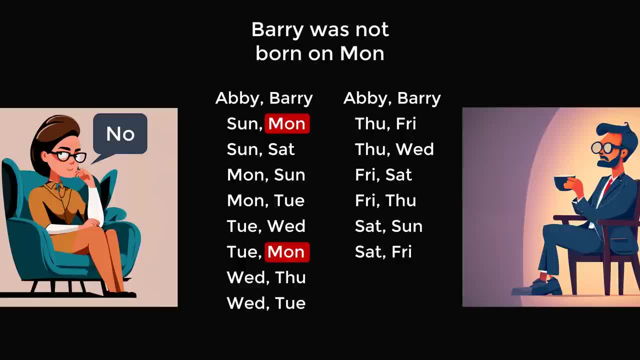 is relayed when Abby replies no. Well, let's think about this logically. Suppose that Abby were born on a Sunday. Abby knows that Barry was not born on Monday, So Sunday comma Monday is not possible. If Abby were born on a Sunday, she would then have been able to deduce that Barry 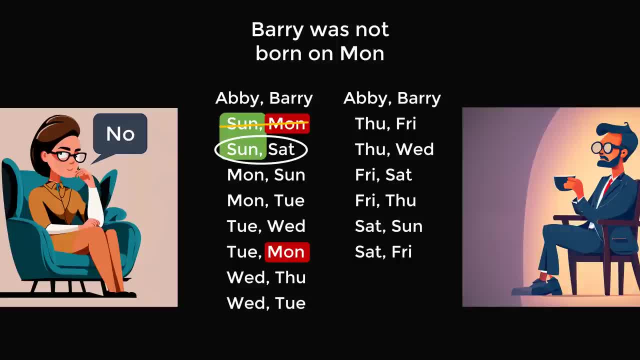 was born on a Saturday, But we know that she said no, So it could not have been the case that she was born on a Sunday. Similarly, if Abby were born on a Tuesday, she would then have been able to know that Tuesday comma Monday is not a possibility. She would eliminate that because. 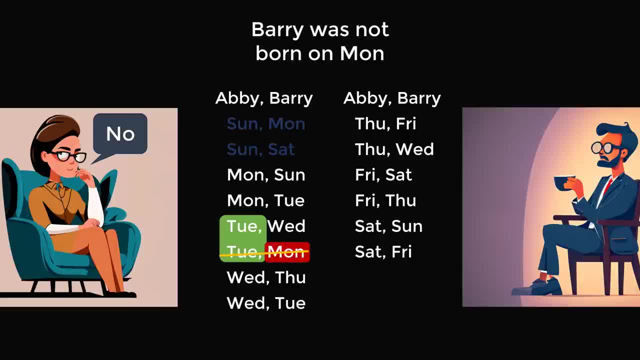 Barry was not born on Monday, So she would have been able to deduce that Barry was born on a Wednesday. But since Abby said no, it is not the case that she was born on a Tuesday, So we can also eliminate these possibilities. Since Barry is a perfect logician, he can also follow through. 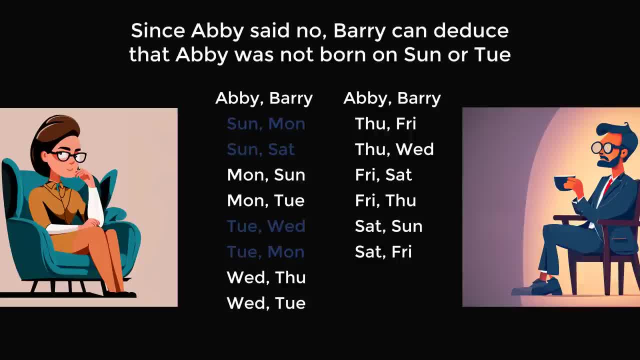 on the reasoning that Abby had, Since Abby said no, Barry can deduce that Abby was not born on Sunday or Tuesday. So Barry then tries to analyze if he can deduce when Abby was born, But once again we get an answer of no, this time from Barry. So what information does that reveal? Let's go. 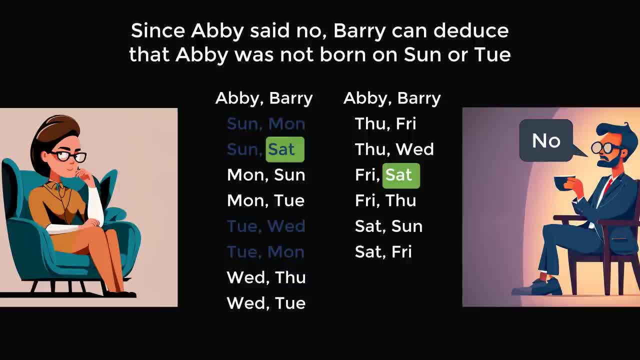 through the following reasoning: Imagine that Barry were born on a Saturday. There are two possible ordered pairs: Sunday, Saturday or Friday Saturday. Now Barry can eliminate Sunday Saturday because he knows that Abby was not born on Sunday. That would leave only the possibility of Friday Saturday. He would be able to. 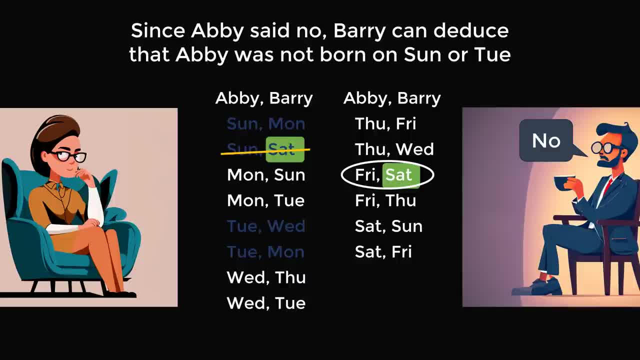 figure out which day of the week Abby was born on, But since Barry said no, we know that this could not be the reasoning, So we can eliminate this possibility. Now let's imagine that Barry were born on a Wednesday. It could either be the order's pairs Tuesday, Wednesday or Thursday Wednesday. 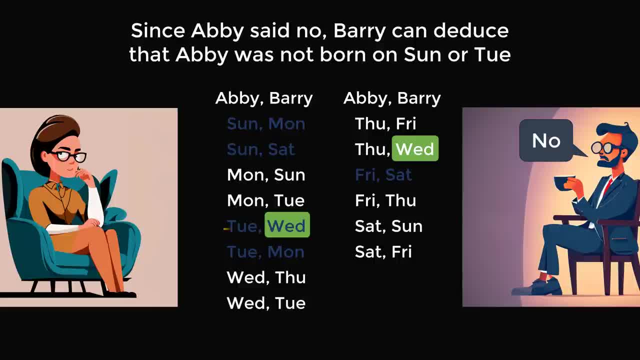 Since Barry knows that Abby was not born on a Tuesday, he could eliminate one of these ordered pairs and he would have been able to deduce the day of the week that Abby was born on. But we know he said no, so this is not the case. We eliminate these possibilities. 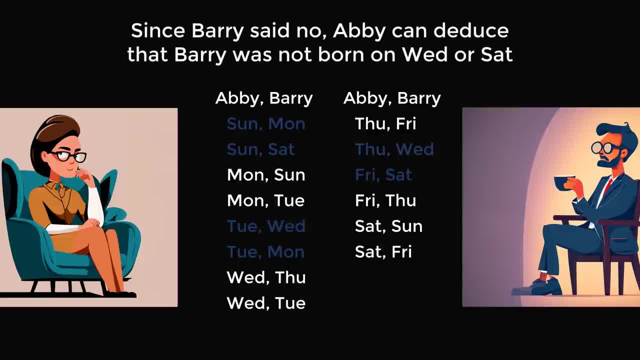 So now the next domino has fallen. Since Barry said no, Abby can deduce that Barry was not born on Wednesday or Saturday. So here's the next step: Abby tries to reason it out and Abby also says no. So what does that tell us? Imagine that Abby were born on a Thursday. It could either be. 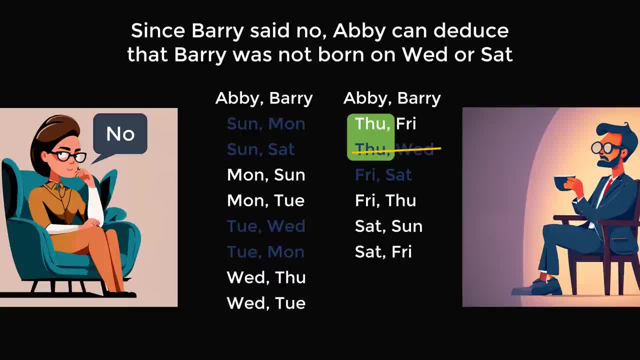 the pair's Thursday-Friday or Thursday-Wednesday, But Abby can eliminate Thursday-Wednesday, which would leave only one possibility. Since she said: no, we can eliminate this case, If Abby instead were born on a Friday, she could again eliminate one of the possibilities, and it 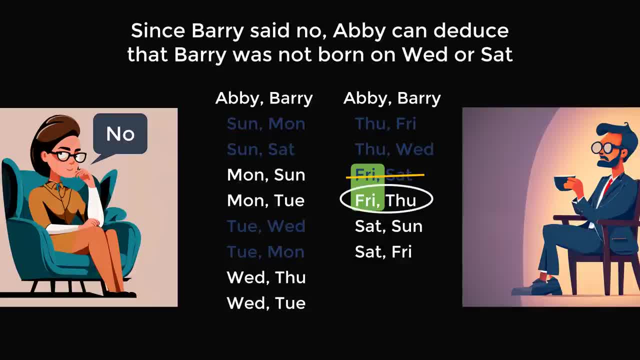 would only be left with one possibility, so she would have been able to deduce it. Since she said no, we can eliminate this case as well. So now, what does Barry reason? Since Abby said no again, Barry can deduce that Abby was not born on Thursday or Friday. So Barry does his deduction. 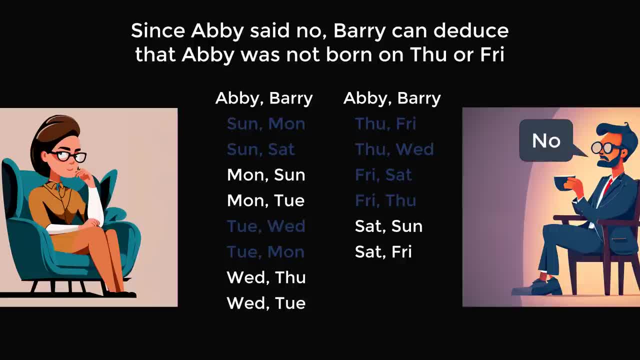 and he once again says no. So now imagine that Barry was born on a Friday. The two possibilities would be Thursday-Friday or Saturday-Friday, but he can eliminate that Abby was born on a Thursday, So he would have been able to figure out the day of the week that Abby was born on. 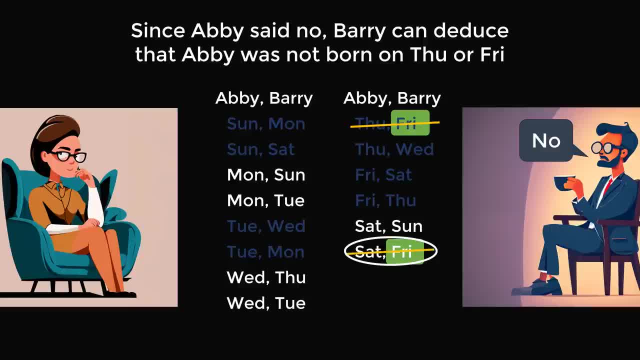 He once again said no, so this was not the case. Eliminate this possibility. Imagine that Barry were born on a Thursday. He could eliminate one of the pairs because he said no. and he could eliminate one of the pairs because he knows that Abby was not born on Friday and he would have been. 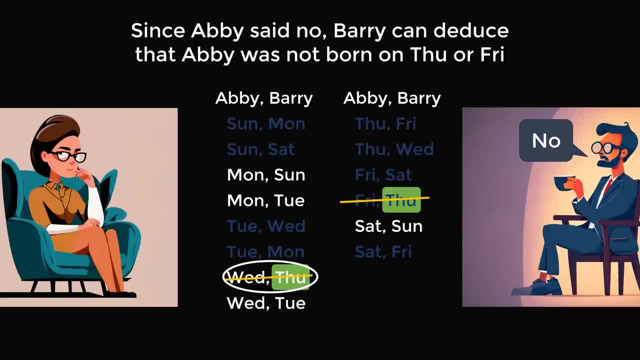 able to figure out the day of the week that Abby was born on. He says no, so we eliminate this possibility. Since Barry said no, Abby can then deduce that Barry was not born on Thursday or Friday. So she's asked again: can you figure out the day of the week that Barry was born on? And again she: 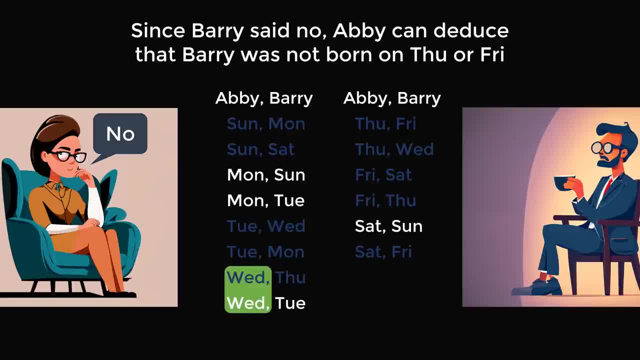 says no. So what happens in this stage? Imagine that Abby was born on a Wednesday. she could eliminate the possibility that Barry was born on Thursday-Friday. She gets a chance to eliminate the possibility that he was born on Wednesday and she reverse the той then should end the. The problem is: 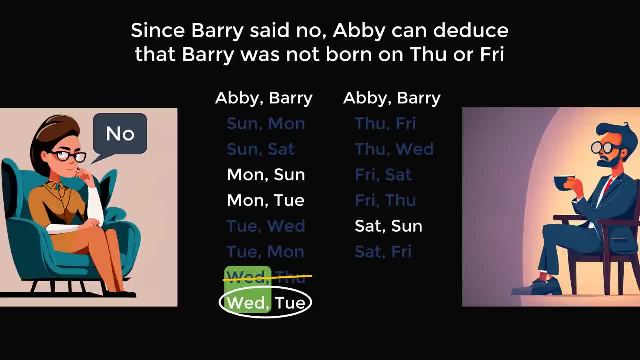 that if Barry was born on the Friday next week- or was he born on Sunday at all times, or so the way Thursday, leaving only one possibility, Since she said no, we can eliminate this case. Imagine that she was born on a Saturday. She'd be able to eliminate that Barry was born on a Friday. 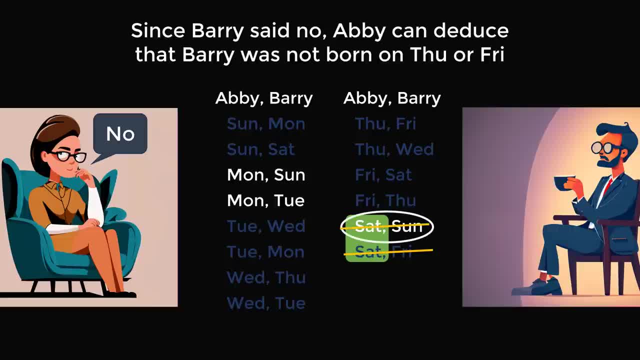 leaving only one case. But she says no, we can eliminate this possibility. So now we're at this stage, Since Abby said no, Barry can deduce that Abby was not born on Wednesday or Saturday. And at this stage Barry says yes, I know the day of the week that Abby 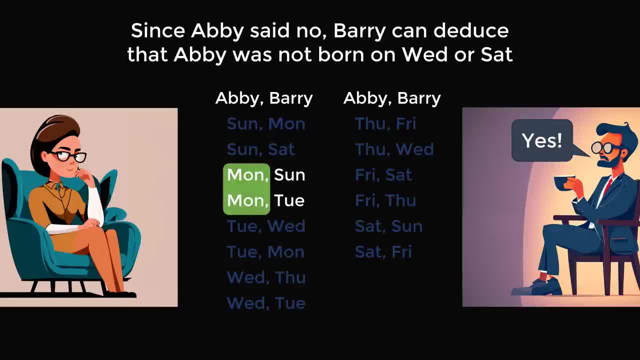 was born on, And we can also deduce that Abby was born on a Monday, So that is the correct answer. We cannot figure out the exact day of the week that Barry was born on, but we know that it has to be Sunday or Tuesday, And that's the answer to this wonderful puzzle. Thanks for making us one.